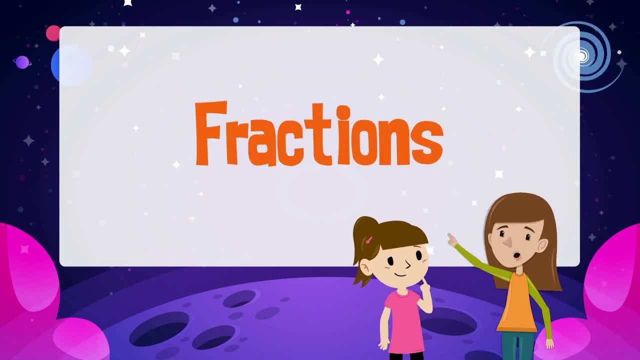 Today, I will teach you about fractions. Fractions are very simple to understand. Well, that's only because you're older and you've been doing math since the dinosaur age. Well, look, I will show you that fractions are really simple. You just have to trust me. 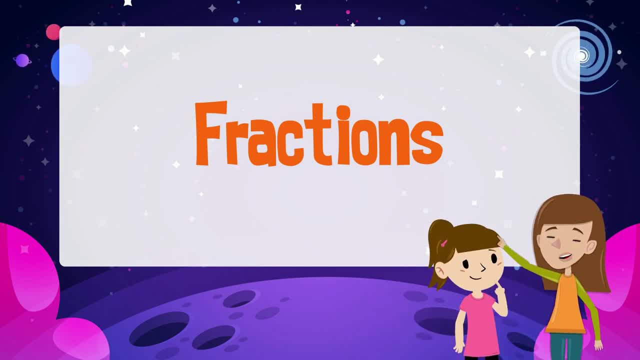 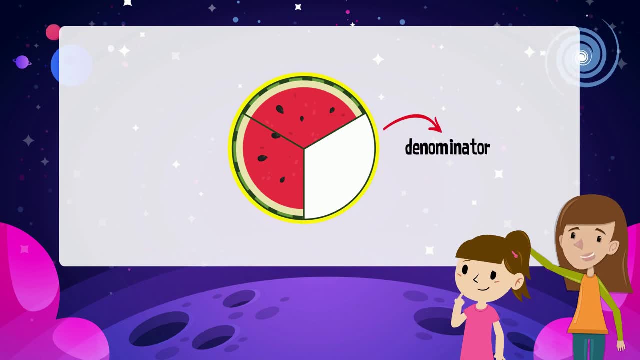 Okay, let's do this before we get to the space station. Fractions are very simple. You need to think of fractions as a part of a whole. The part is the numerator in a fraction and the whole is the denominator: A part of a whole. What does that even mean? 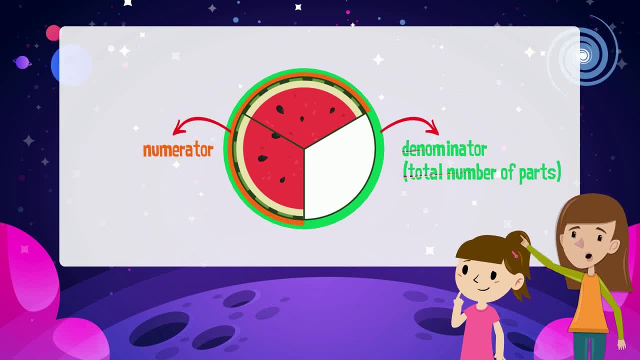 Every fraction has a whole and every fraction has a numerator and a denominator. To find the denominator, we just need to look at how many equal parts our whole has been partitioned or divided into. If you can count fractions, are super easy. How many equal parts do you see here in this fraction? Can you count them? 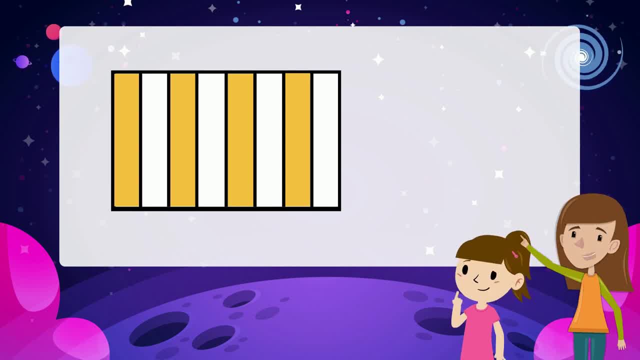 Does that mean I just need to count all the equal parts within the whole? Yes, we can even count them together. Let's see how easy this is. Okay, so I see a total of 1, 2,, 3,, 4,, 5, 6,, 7, 8.. 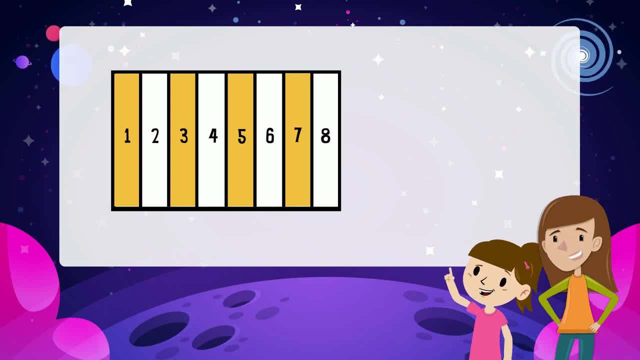 This whole has been divided or partitioned into 8 equal parts. Yes, this fraction has a total of 8 equal parts, so the denominator of this fraction is 8.. The 8 tells you how many equal parts are within a whole, in a fraction. 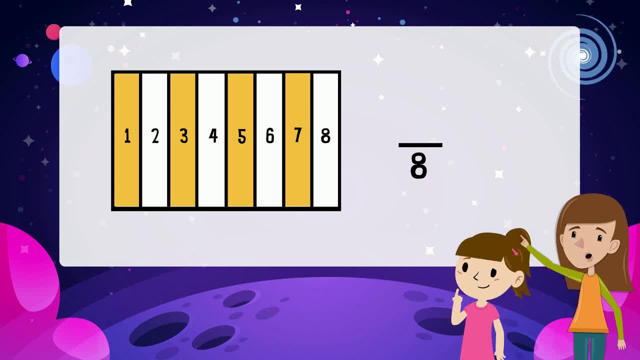 And how about the neuro-ruminator? You mean the numerator? Yeah, that thing. Well, that is even easier. The numerator tells you how many parts you have. That is often represented in a fraction by what is shaded. How many of the parts do you see shaded? 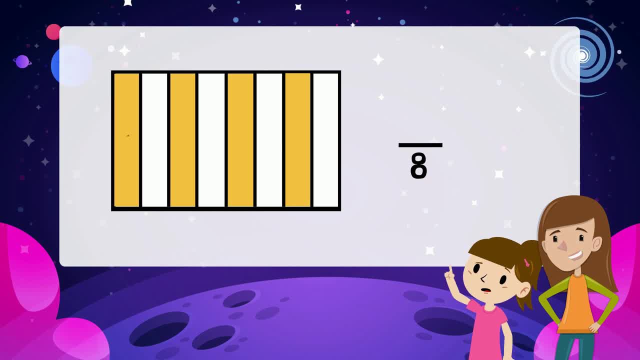 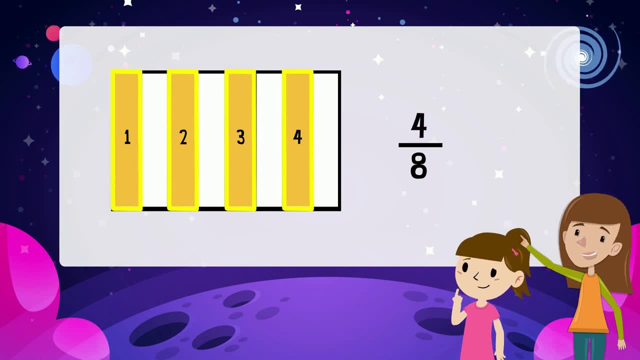 Let's count them together. Okay, so I see a total of 1,, 2,, 3, 4 parts that are shaded. Good, that means that our numerator is 4.. Our fraction is 4 eighths. 4 out of 8 equal parts are shaded. 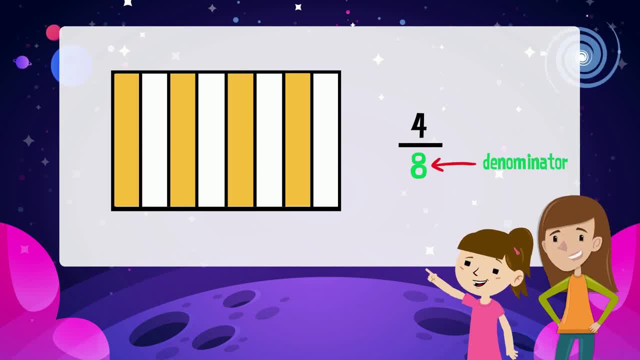 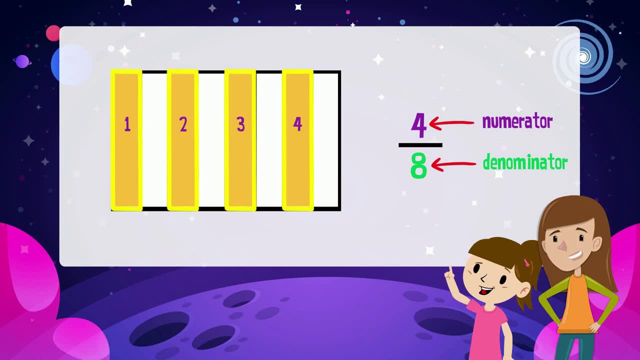 Do you remember where each number came from? Yes, the denominator or number in the bottom is the total number of equal parts that are within our whole, And we found our numerator by counting the total number. So we have 4 equal parts. Well, that was easy. 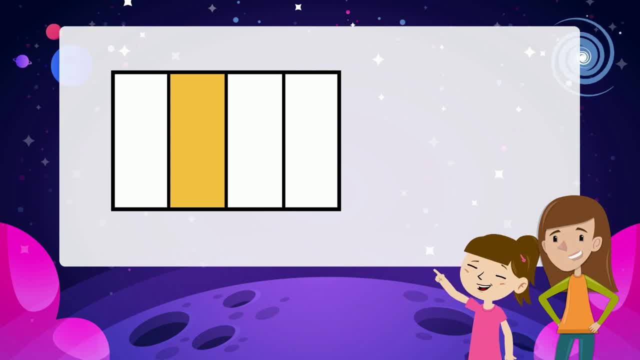 Let me give you another fraction. Okay, so I see that there are a total of 1,, 2,, 3, 4 equal parts. So that is our denominator, or the bottom number in our fraction. Good, and how many of those parts are shaded? 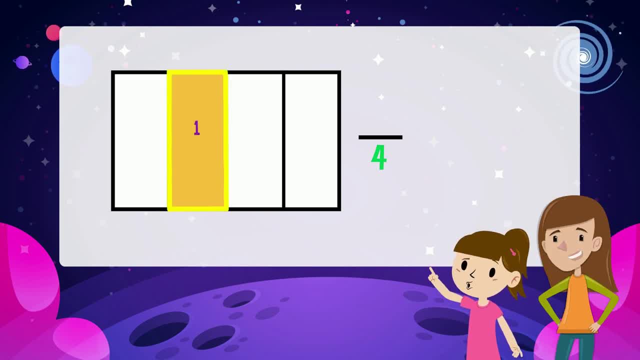 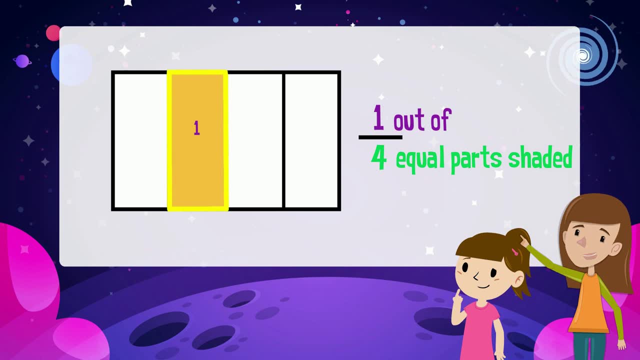 There is only one part that is shaded, So the fraction represented here is 1 fourth. 1 out of 4 equal parts are shaded. Awesome. now I want to challenge you: What part of the fraction is not shaded? Does that mean I need to count the total number of parts that are not shaded?